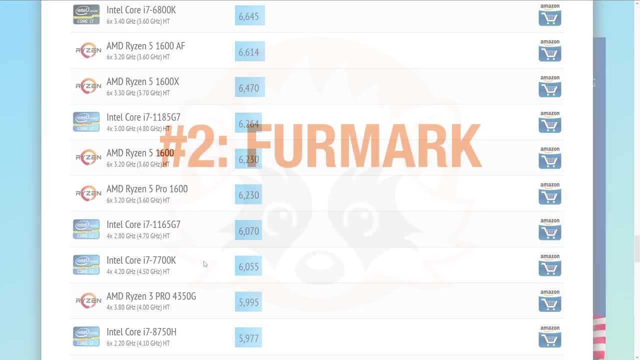 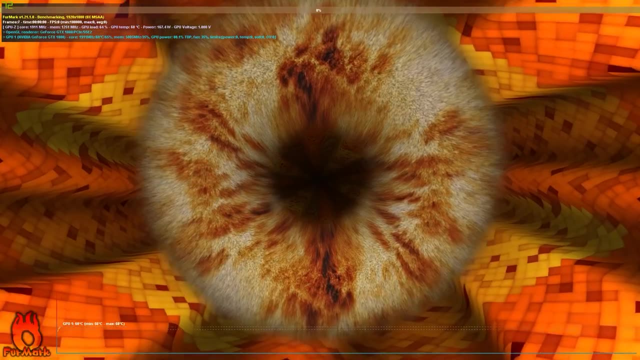 stacks up against others, For instance on CPU Monkey. The second benchmark program on our list is Furmark, aka the furry donut. It is well known for being a stress test that literally burns your GPU If it is overclocked heavily, of course. 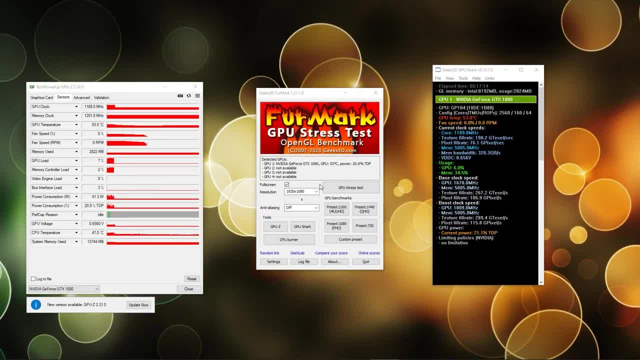 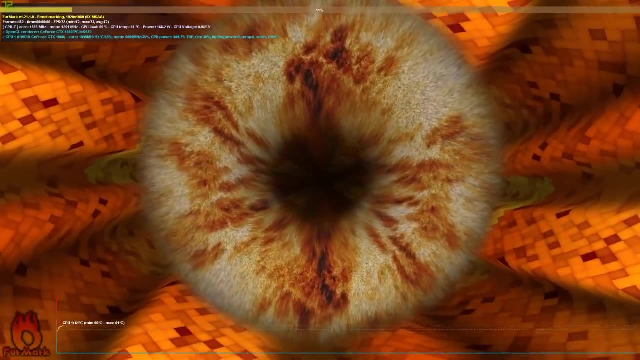 Next to the stress test, Furmark has the option to benchmark your GPU. The results you will eventually get scale with the chosen resolution. So be careful which resolution you're choosing for comparing your results with other GPUs. The most common preset is, of course, 1080p, followed by 1440p- Again a higher score. 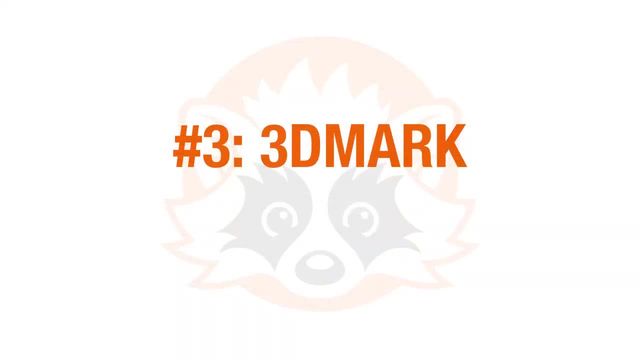 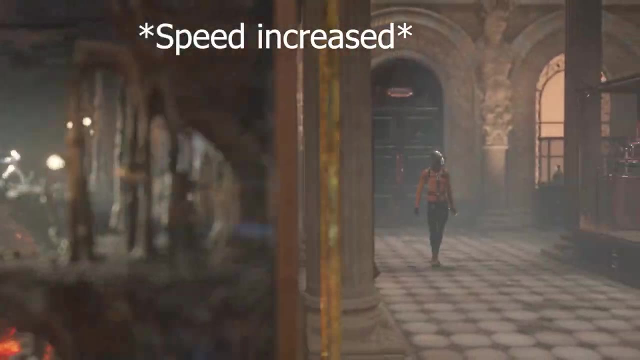 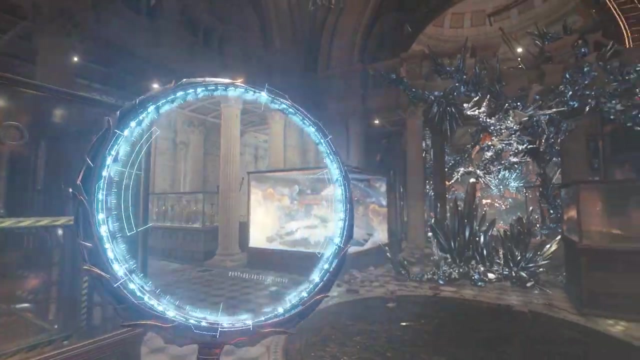 indicates better performance. Number 3 on our list and with a 3 in its name is, of course, 3DMark. 3DMark has a free and also a paid version. You can download a free demo version on Steam and use the so called Time Spy benchmark within 3DMark, What is appreciated by most beginners. 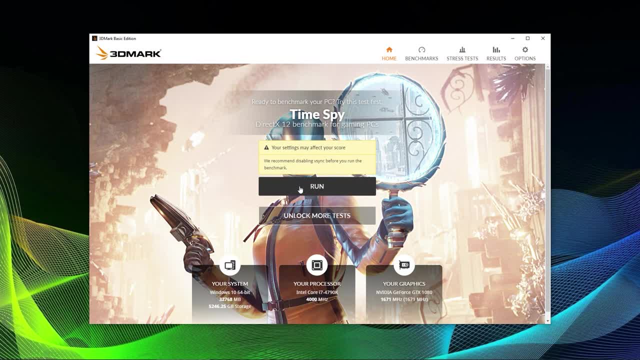 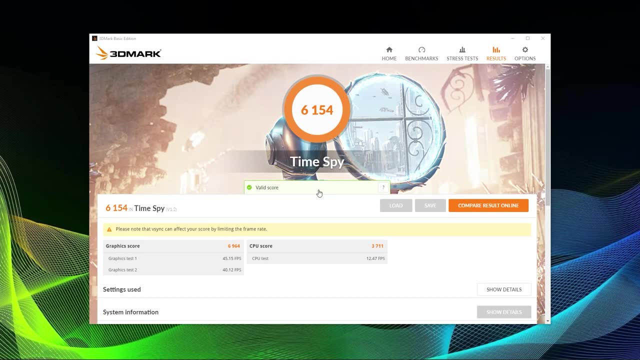 is the fact that no settings have to be chosen. It's a simple one click benchmark. After running a couple of scenes, you will get an end result with a score. What we find most compelling about 3DMark is that your overall score considers CPU and GPU. 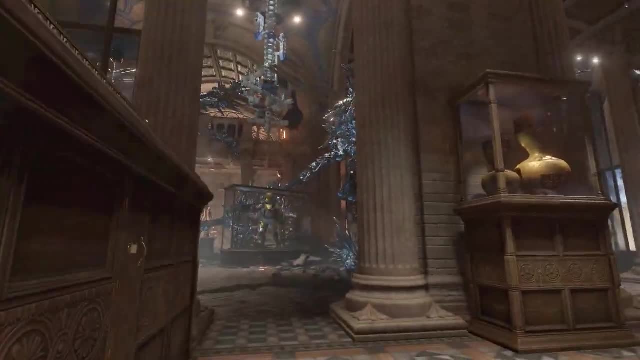 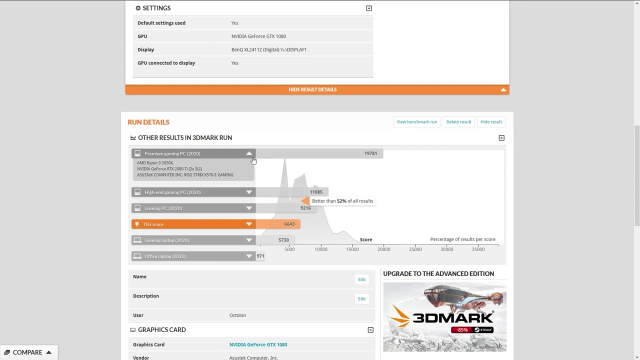 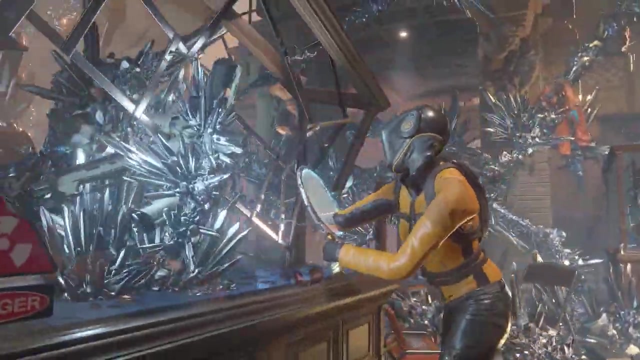 performance and ranks your system with all other systems worldwide that have completed and reported the benchmark results. So it's easy to see where your system ranks and you can get inspiration from other systems in case you're planning an upgrade. It's needless to say that before and after an upgrade of any important component, you can see the effects. 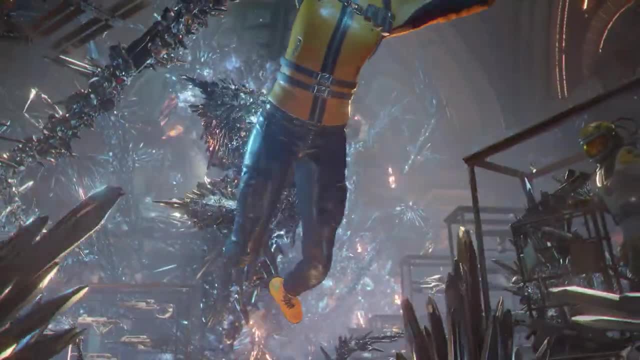 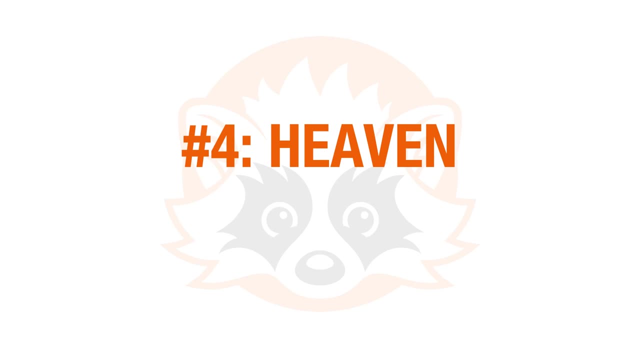 coming from it. It goes without saying that this is the case for almost all benchmarks. Number 4 on our list is the heaven benchmark. Heaven benchmark by Unigine has been around for ages and is still a very popular tool to measure your GPU performance. It has a ton of settings. 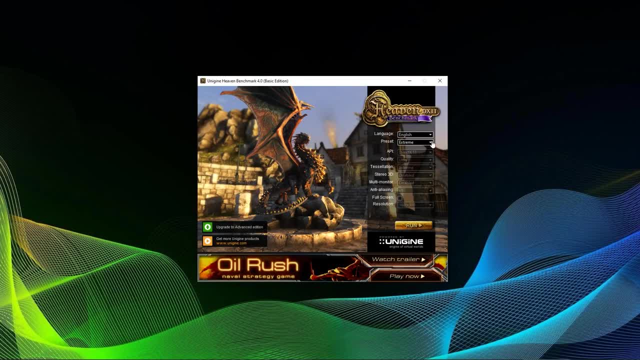 you can alter, and you should be able to distinguish between what the settings do and what they don't do, Because the score you will receive at the end does not scale with resolution or details you select. So with some of them it would be harder to get a better score, For example, if you had a 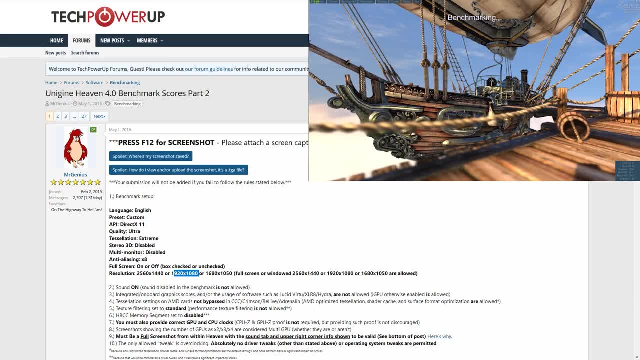 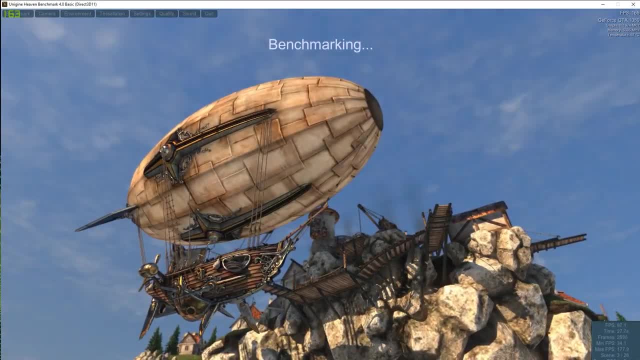 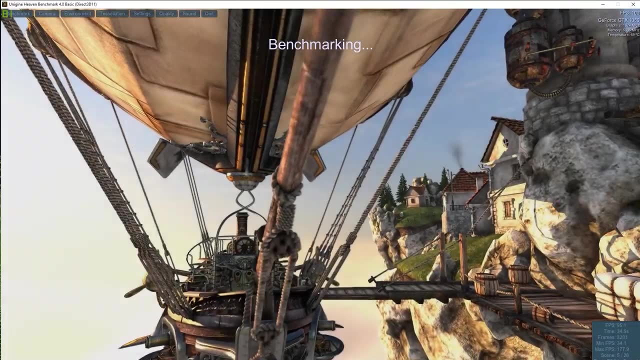 what settings to choose. you may consult the TechPowerUp forums, which has a default settings recommendation to be able to compare your results with others. For convenience, we have linked the discussion thread with recommendations and, of course, also results for comparison in the video description. Finally, it should be noted that Heaven is especially popular amongst overclockers. to 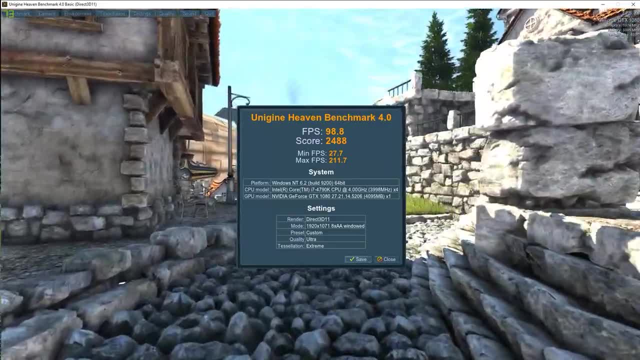 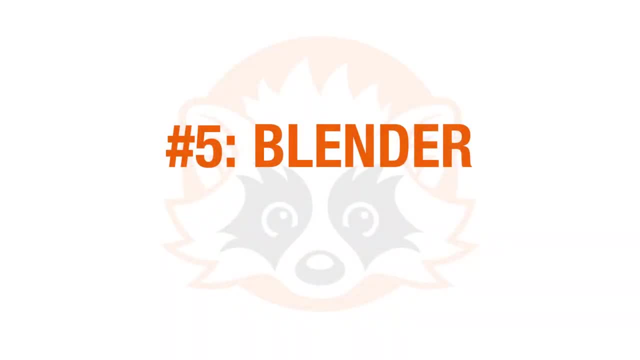 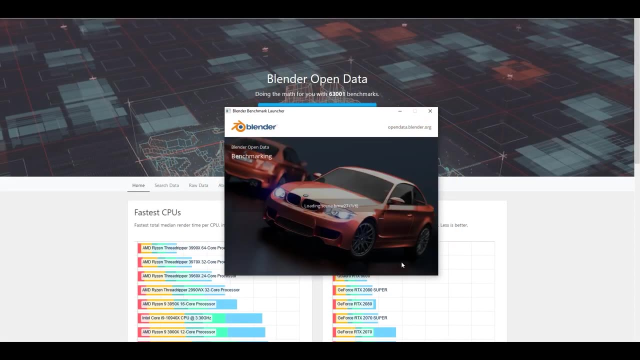 see whether their GPU is stable. You can use it to stress test your GPU like you do with Thermark. Caution should be exercised, though. Number 5 on our list is Blender Open Data. Blender Open Data is using your CPU and GPU to render images kind of similar to Cinebench. 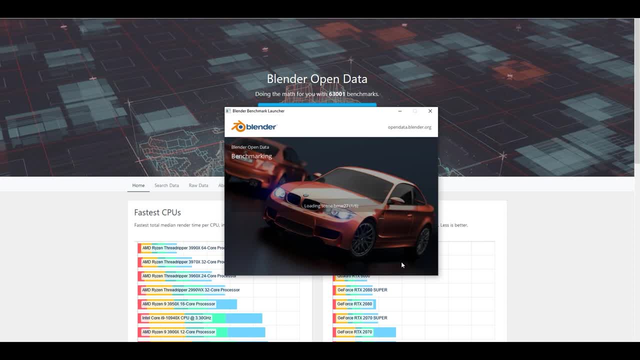 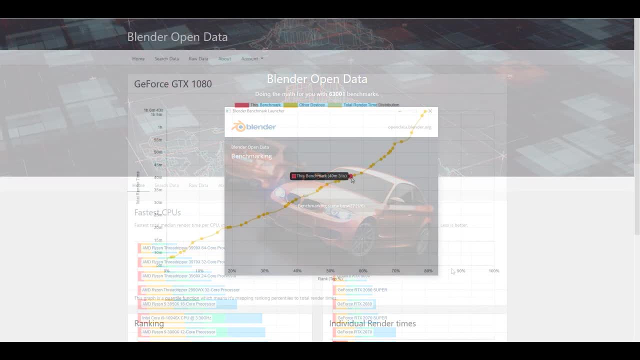 The good thing is that it is also a free out of the box tool that will eventually present you with render times that will be used to show where you rank against other devices. Obviously, a lower score, meaning render time, is better for this benchmark. 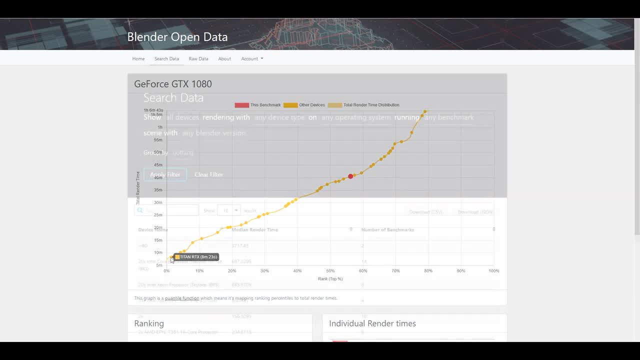 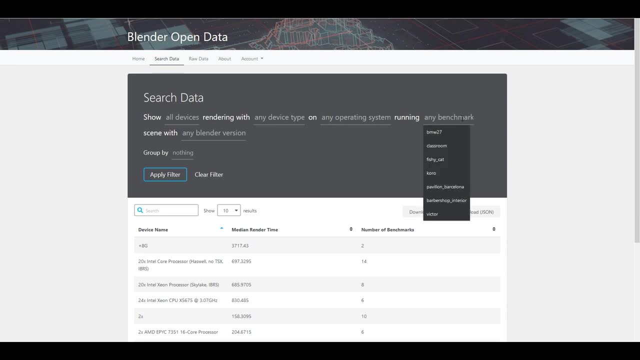 The neat additional feature from Blender is the data that you can search through Meaning. you can specifically look for certain operating systems, devices and even only certain images and their respective render times. Even though we finished the top 5 list of free benchmarking tools, we won't let you. 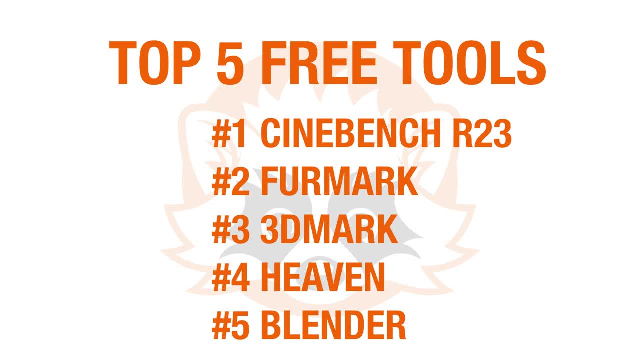 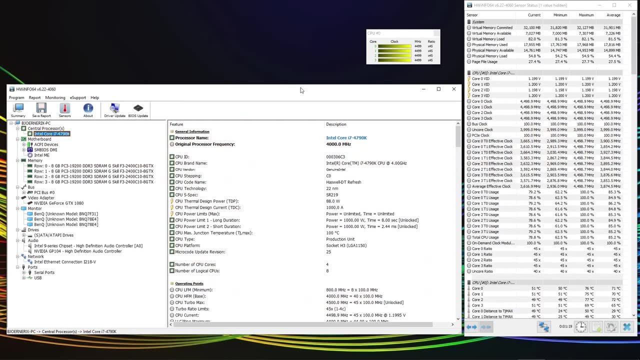 go before we give you a few bonus tools that are also free and should not be missing on your system. While running benchmarks, you better keep an eye on utilization and, of course, the temperature of your components. We highly recommend HardwareInfo, which is also linked in the description of the video. 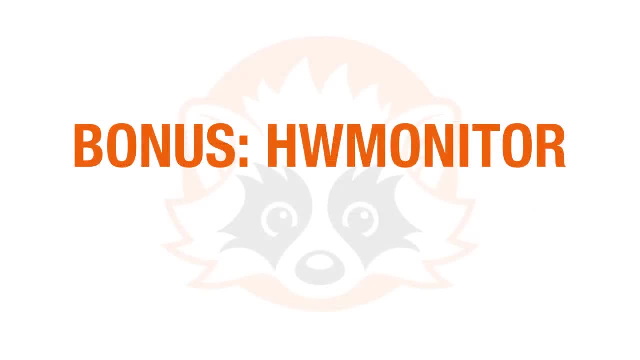 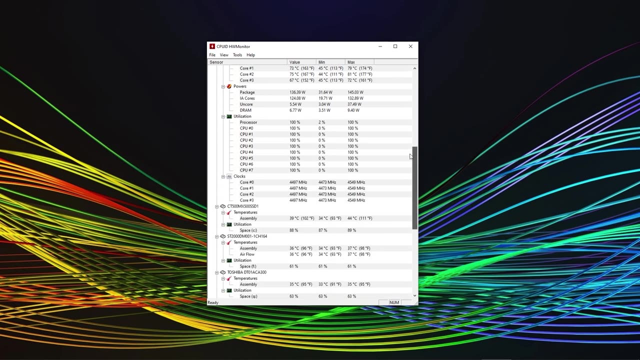 The next free tool is Blender. The next free tool we also recommend is HWMonitor. It is not as comprehensive as HardwareInfo, but still has all the major information you are ever going to need. So if you don't need all the information, HWMonitor is the way to go. 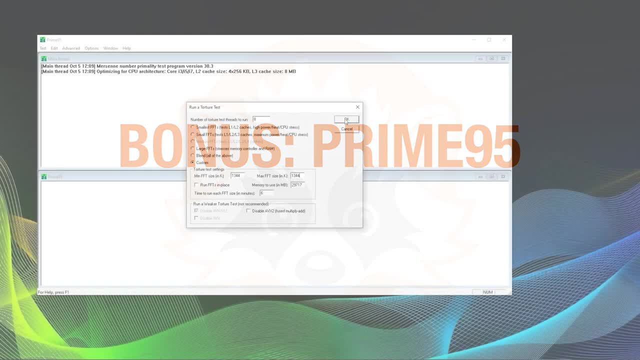 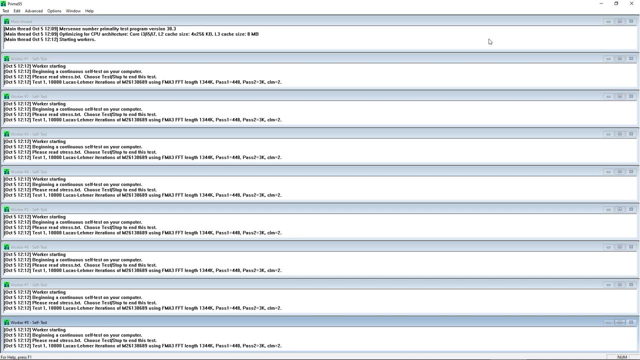 And last but not least, we highly recommend Prime95.. With Firmwork and Heaven, we presented two tools to stress test, or rather test the stability of your GPU. For testing the stability of your CPU, we recommend Prime95. A couple of hours of running Prime95 would be enough for you to be able to test the. 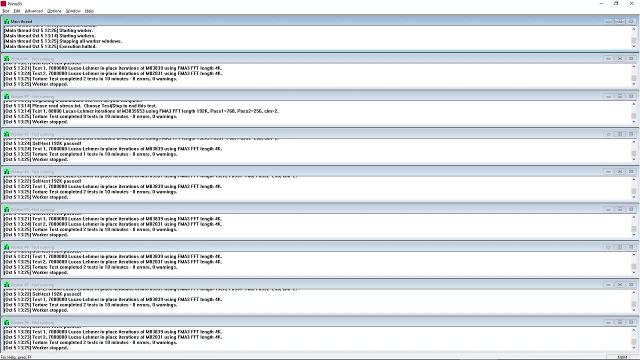 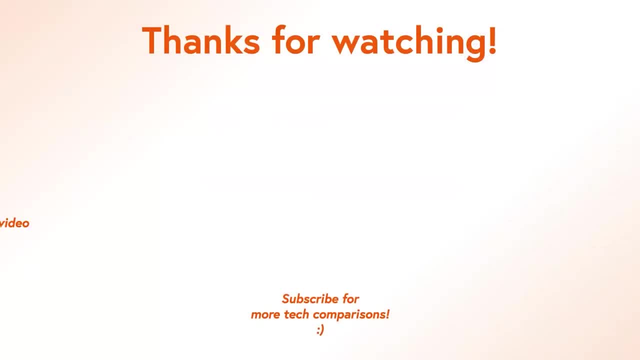 stability of your GPU. Prime95 won't cut it, though it is recommended to run it for 6-10 hours. That is the last tool we wanted to recommend. Do you have any other recommendations? Leave them in the comment section down below.